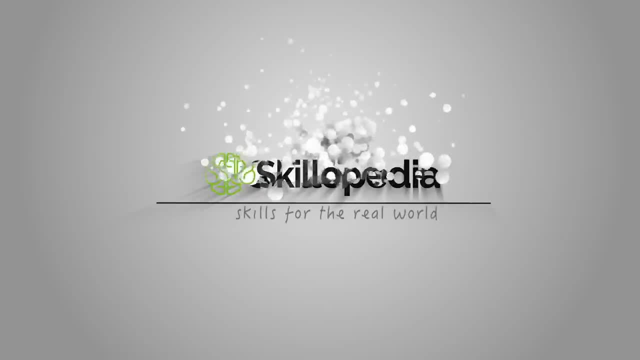 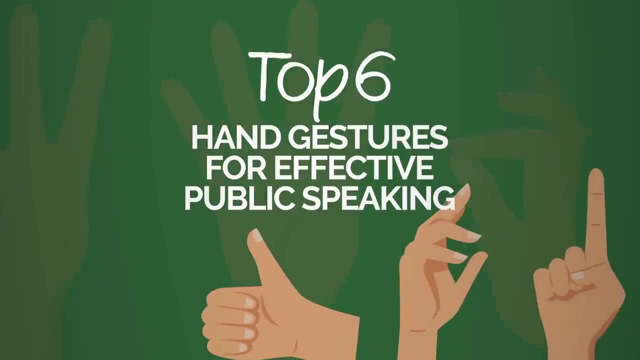 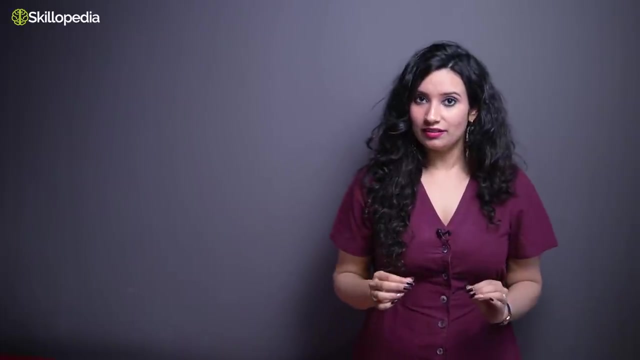 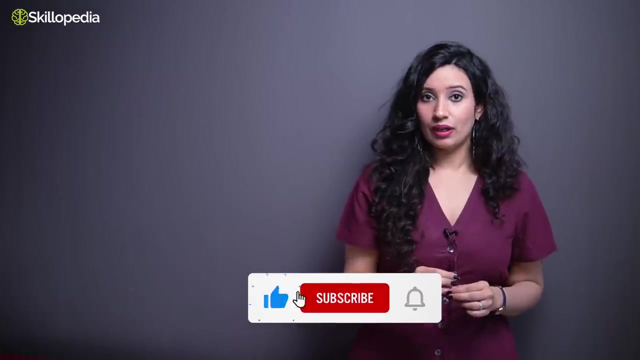 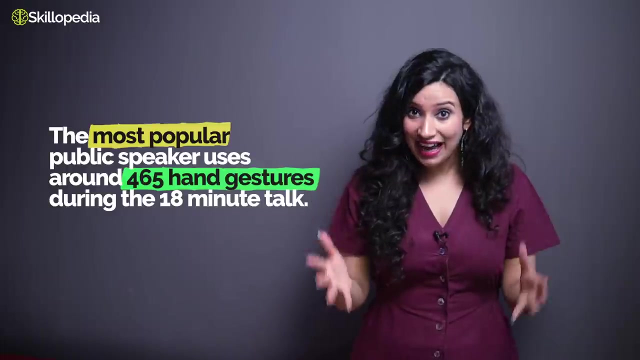 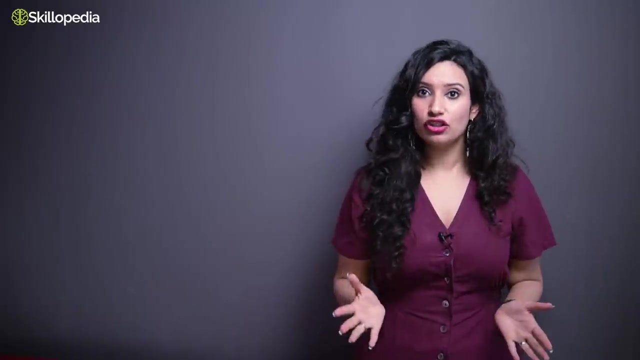 Do you know that the least popular public speakers use an average of 272 hand gestures during the 18 minute talk, Whereas the most popular public speakers use an average of 465 hand gestures in an 18 minutes talk? That's almost the double, and this fact completely. 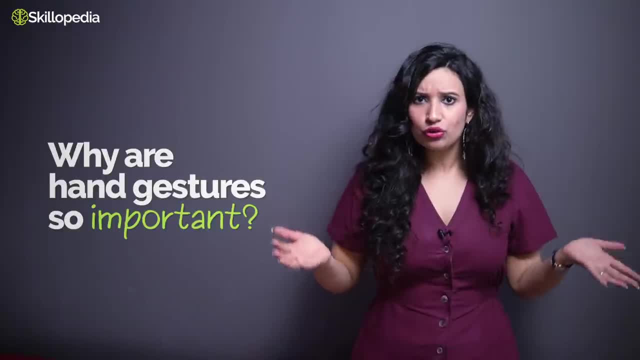 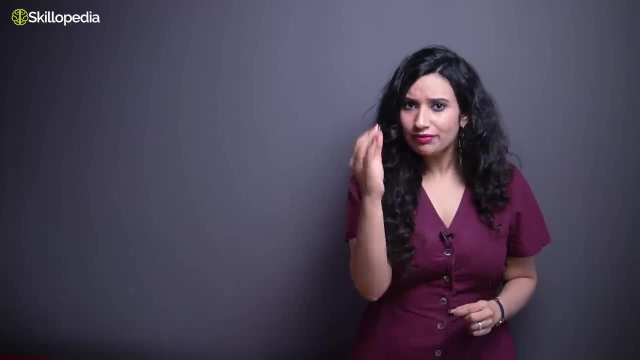 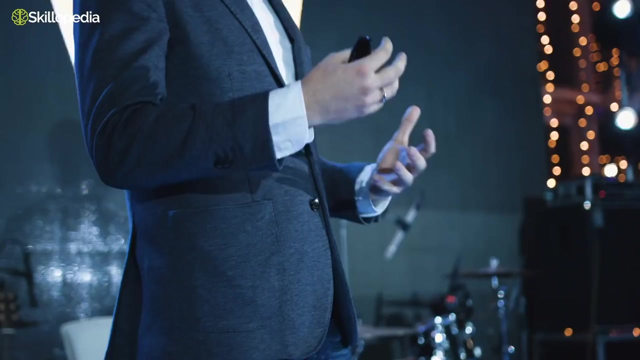 shocked me and made me think: why are hand gestures so important And what are the most popular hand gestures? I also thought of how can everyone use their hand gestures to deliver an effective talk. So what I did is I observed some well-known public speakers and then created 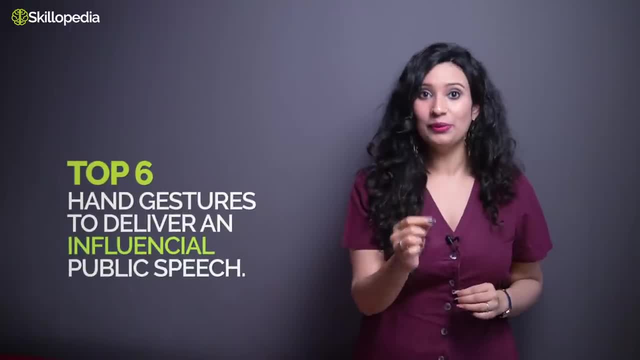 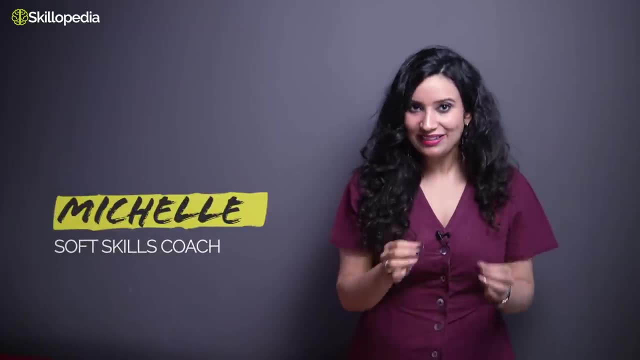 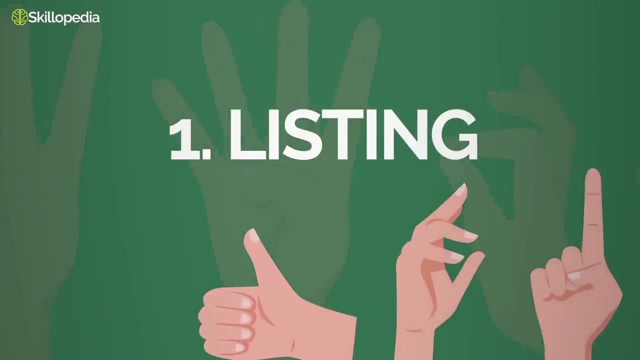 a list of top six hand gestures that can help you deliver an influential public speech. So this is Michelle, and you're watching me on Skillopedia, the place to learn skills for the real world. So let's begin with the first gesture. So the first gesture that I'm going to 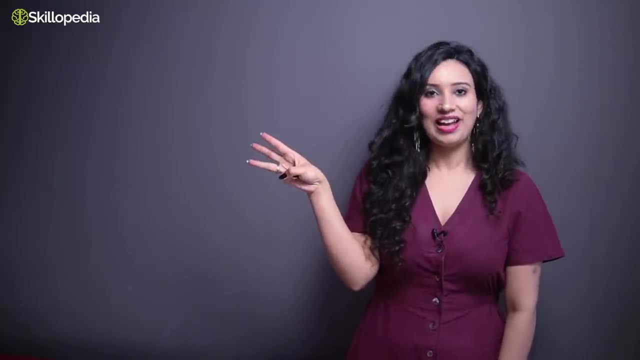 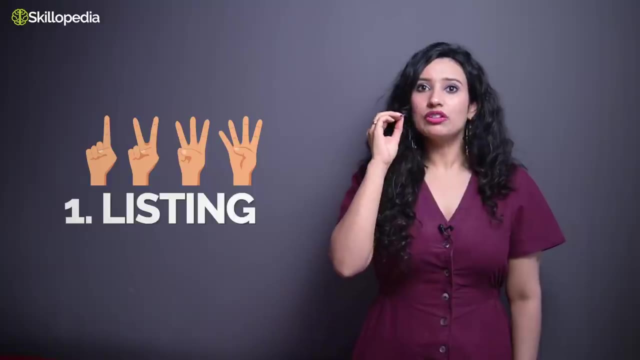 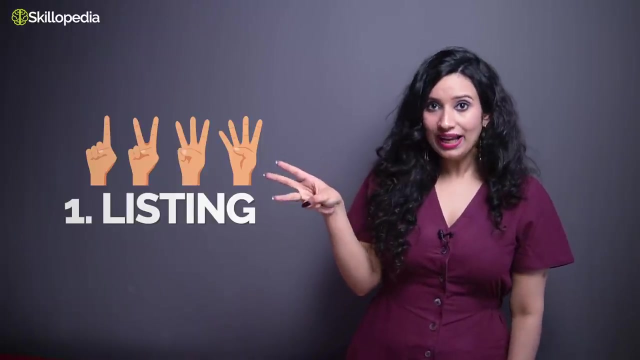 talk about today is mm-mm-mm. Well, do you think? can you guess what I mean here? I mean listing. The easiest and most basic hand gesture is listing. Anytime you say a number, you can list it with your hand. This adds movement and warmth to your body language and also. 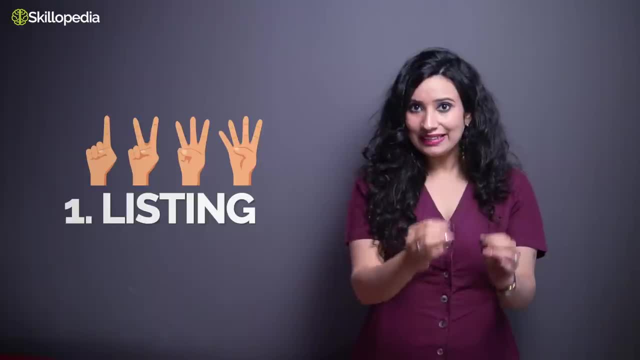 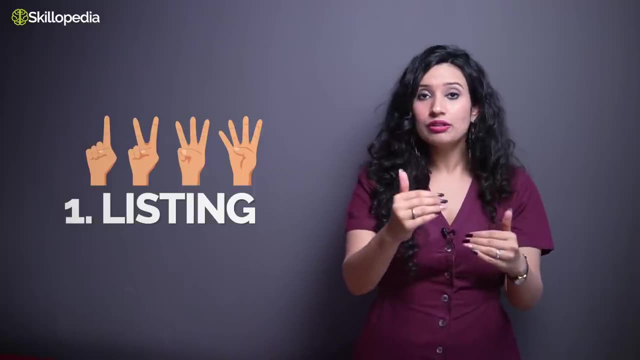 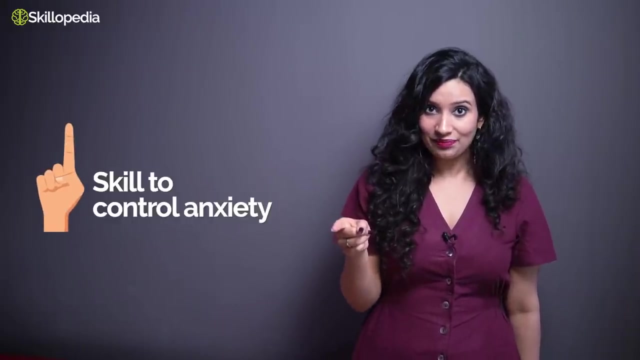 attracts the listener's attention. So let's see an example of how you can use this gesture in your speech. So I know you have the followingrand. you're delivering a speech on why and how to deliver a good public speech. For this you can say one. you need the skill of controlling anxiety. 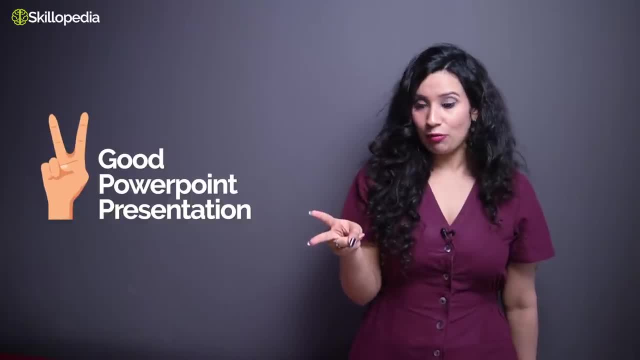 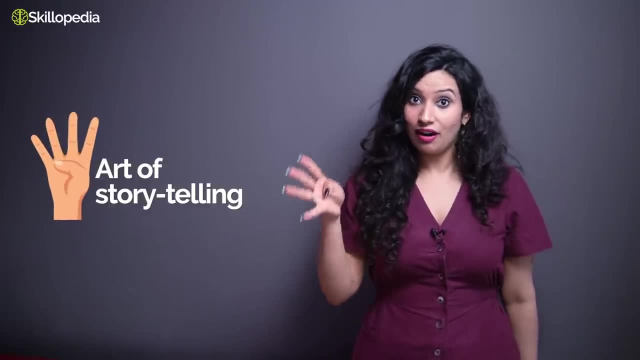 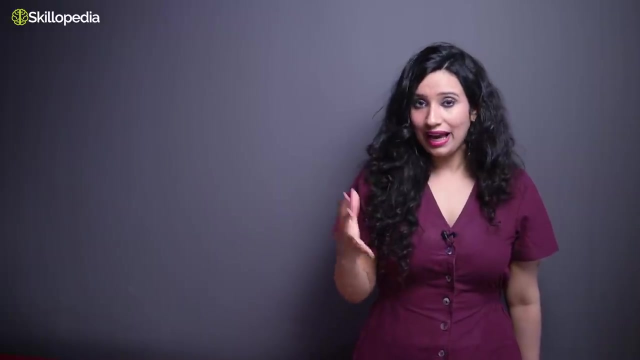 Second, you need the skill of creating good PowerPoint presentations. and third, the skill of maintaining eye contact and forth the list, the art of telling stories and, lastly, using humor. So what you just noticed is I used my hand to draw your attention, So the 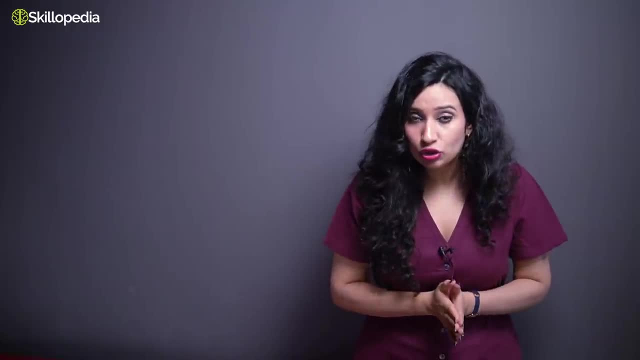 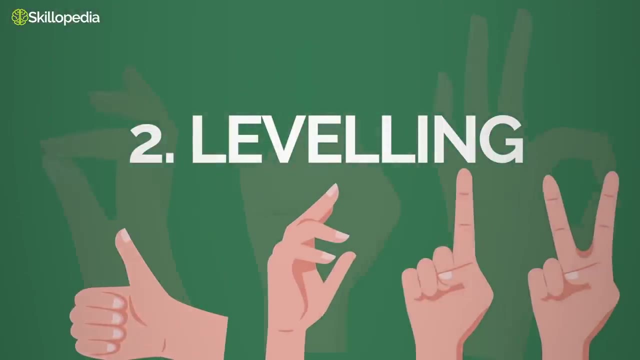 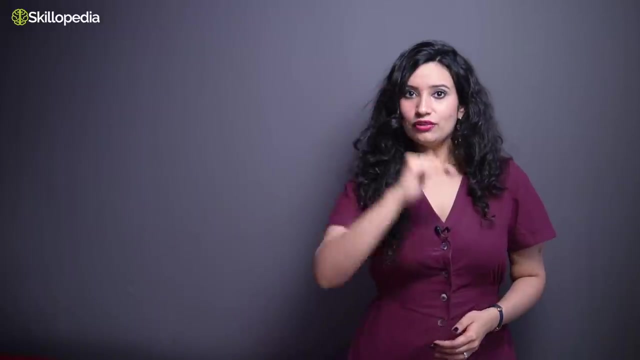 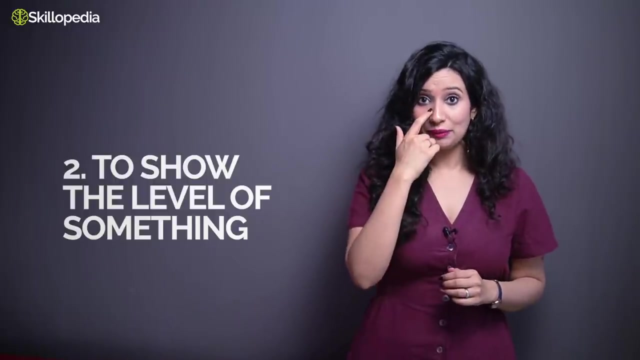 next time you are adding any numbers in your presentation, make sure that you use your hands to do the listing. The next useful gesture is to show the level of something. So this is a really easy one and can be used literally to show someone what level something is. For example, if something 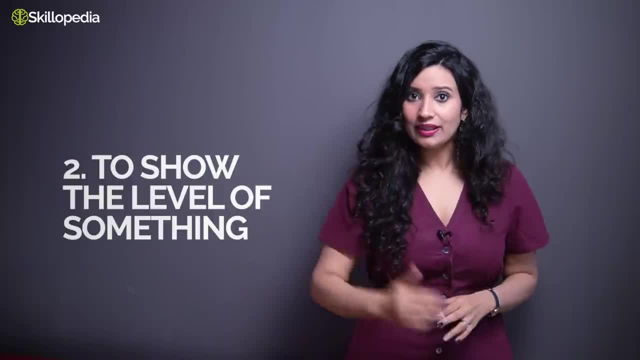 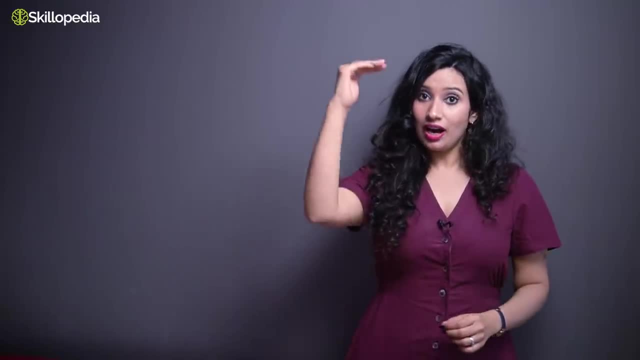 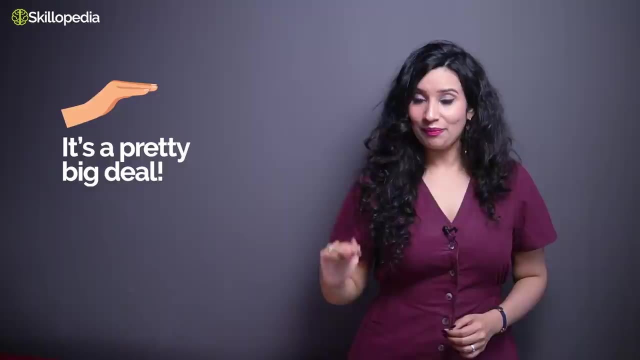 is high or if something is low. you can use this to indicate how big or small something is or where someone stands. Let's look at an example. you can use the high version like this for saying something like it's a pretty big deal. or you can use the low version by: 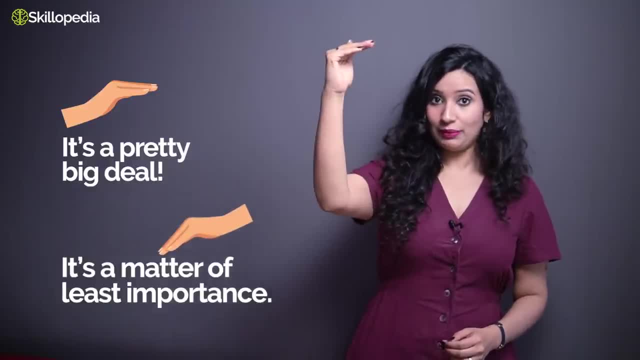 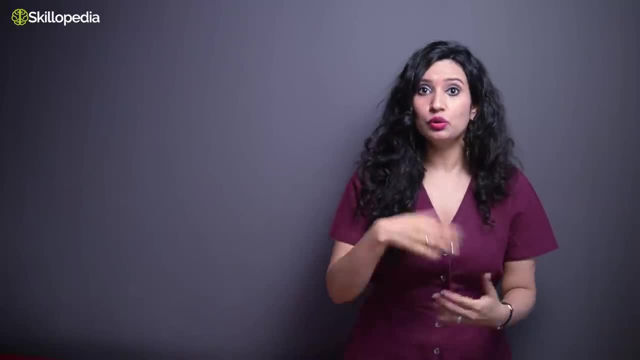 saying it's a matter of least importance. So it's a pretty big deal and it's a matter of least importance. Not only that, you can use this as an alternative to listing as you talk about different stages. For example, you could say in a speech: we start with the. 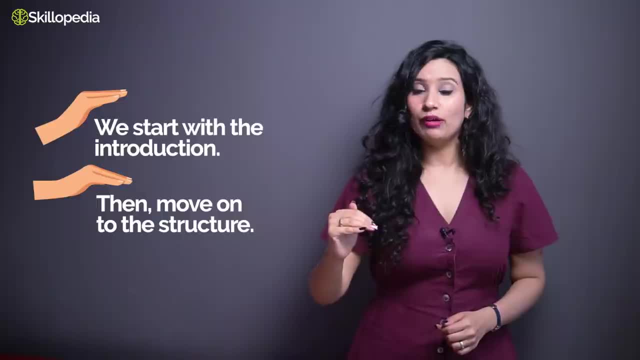 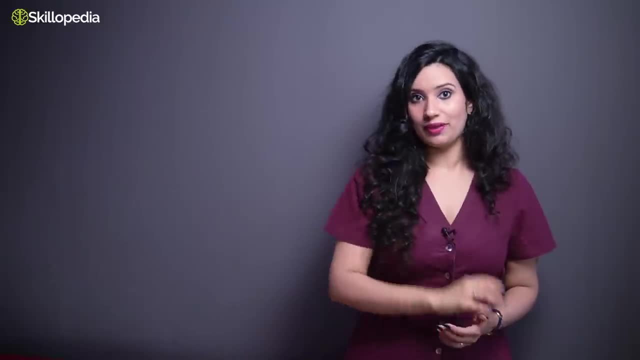 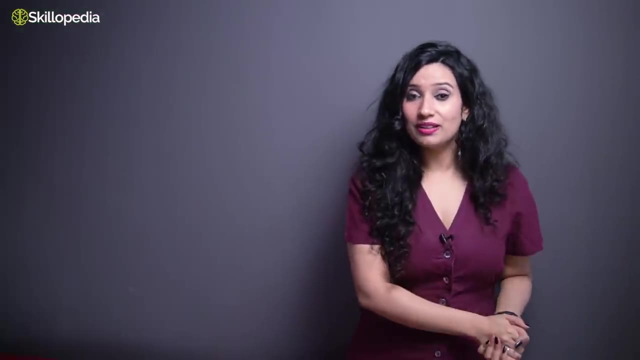 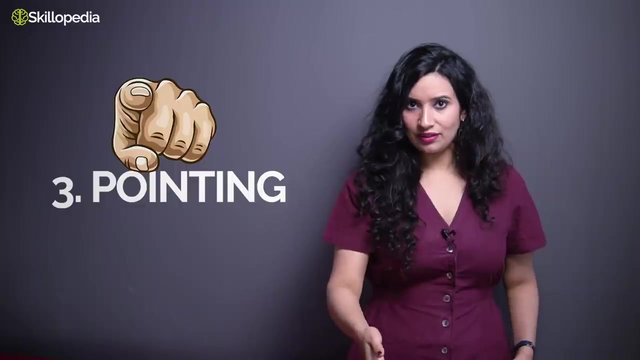 introduction, then move on to the structure and we end with the conclusion. So here I've used my hand to show the level or the structure of something, and next up is the very popular hand gesture, which is pointing gesture. So you didn't expect this to be on the list- and 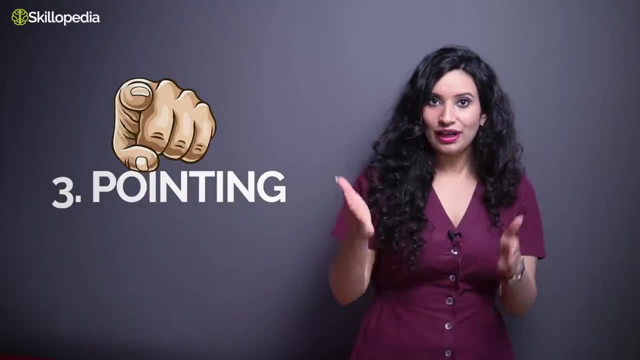 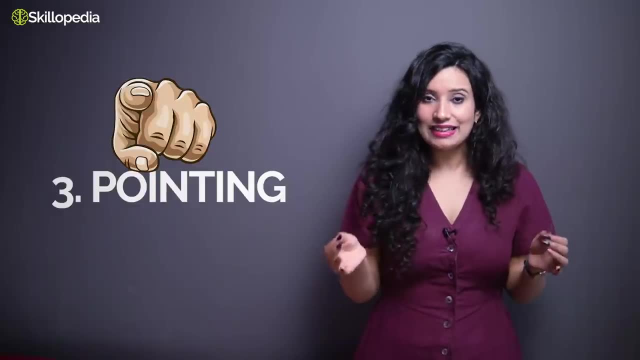 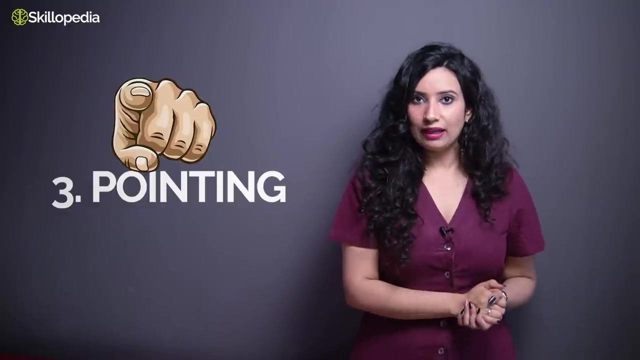 you might be confused That is it positive or negative? Well, I would say that this one should be used with caution, because normally people don't like to be pointed at. It can seem as if you're accusing them. However, you can point to get someone's attention or literally to make a point. For example: 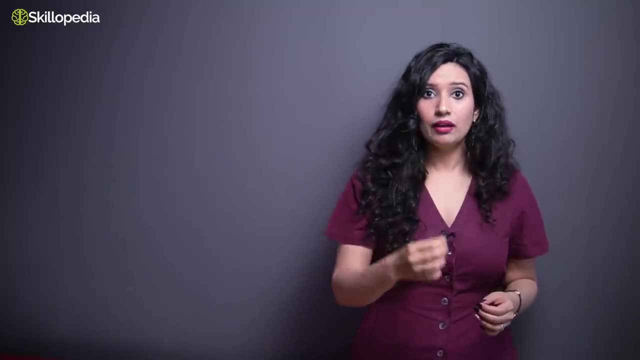 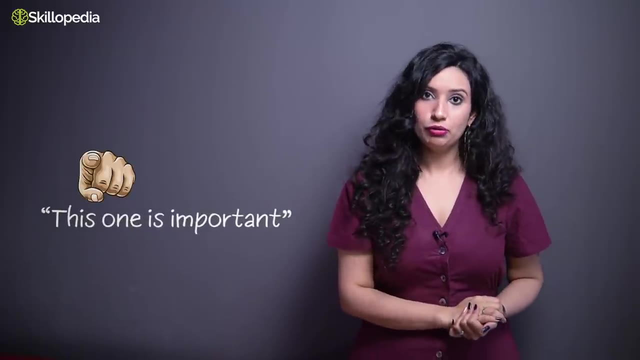 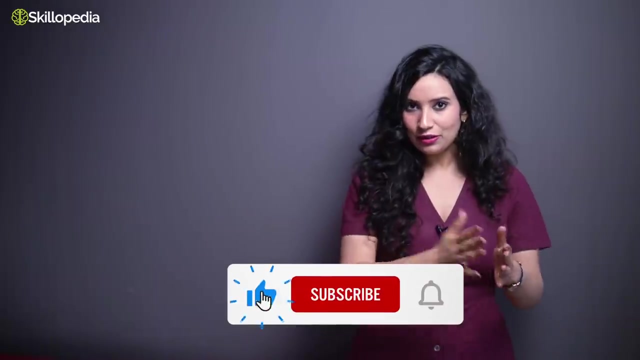 this gesture goes very well along with saying something. like you know, I just remembered something important. or you could say this one's important, or you could use pointing when you want to say let me tell you something, Alright, so here we looked at, we've looked. 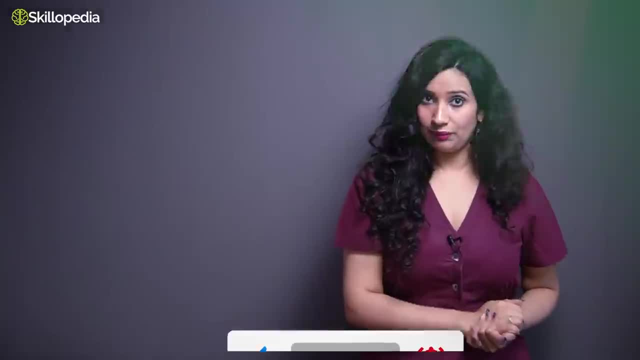 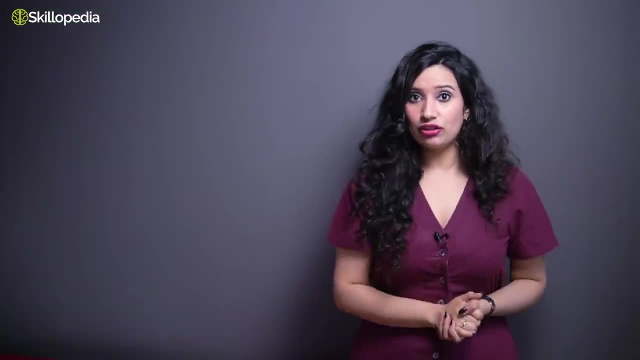 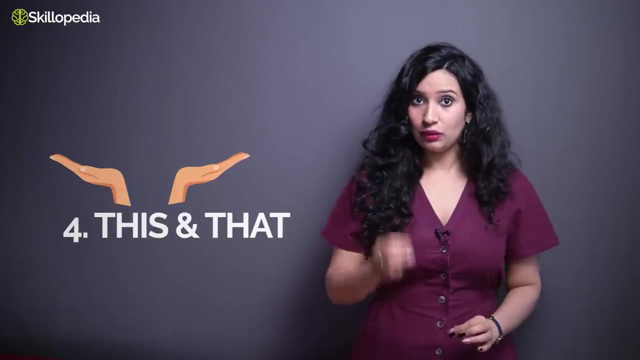 at three hand gestures and now we're going to look at the fourth one. So the next hand gesture is this and that Whenever you want to separate two different ideas or things that you're saying, you can use your hands to represent that, For example, 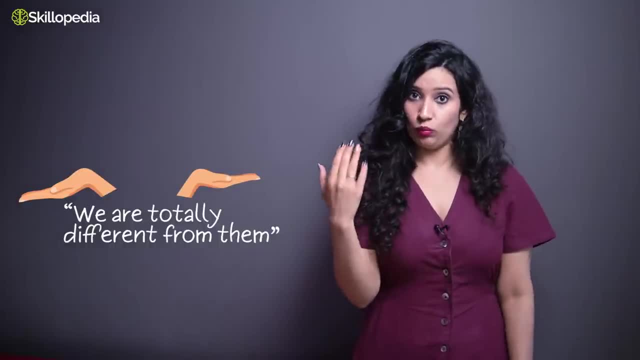 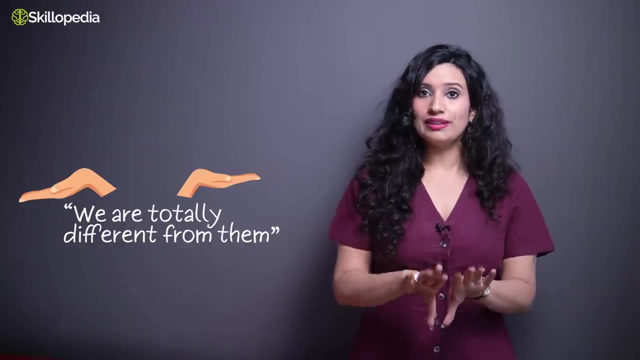 totally different from them, Using my left hand when I say we and my right hand when I say them. So this is a great way to put distance between two things and show that these are two separate things or two separate ideas. So once again you could say: you are. 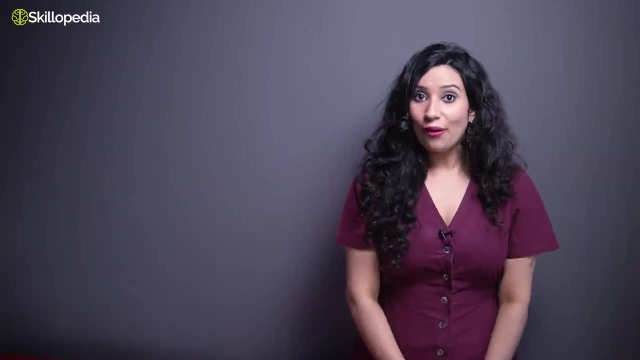 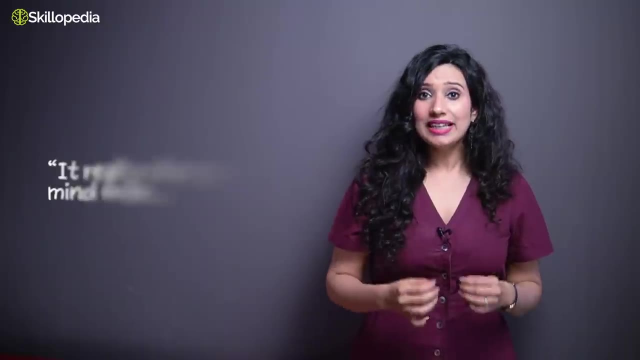 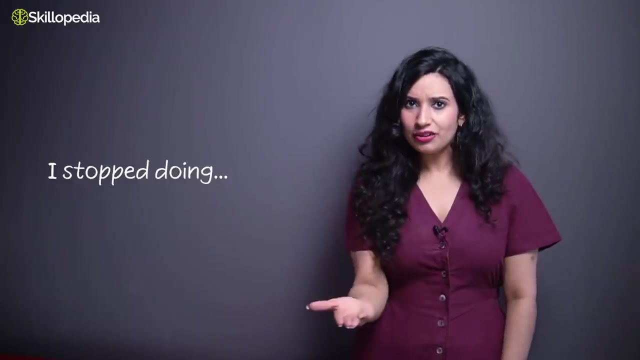 we are totally different from them. Also, you can use this gesture to show a change. It can be used along with this example. it really changed my mind from positive to negative. Or you could say: I stopped doing hard work after I learned about smart work. So just 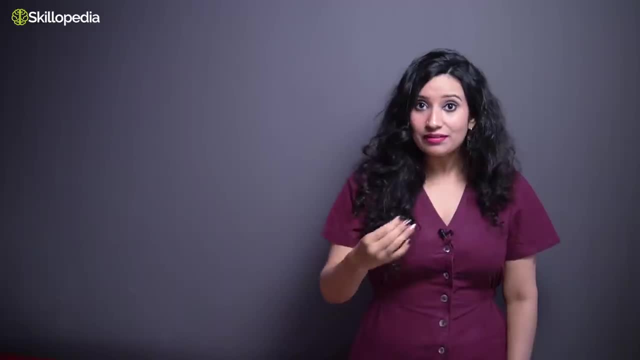 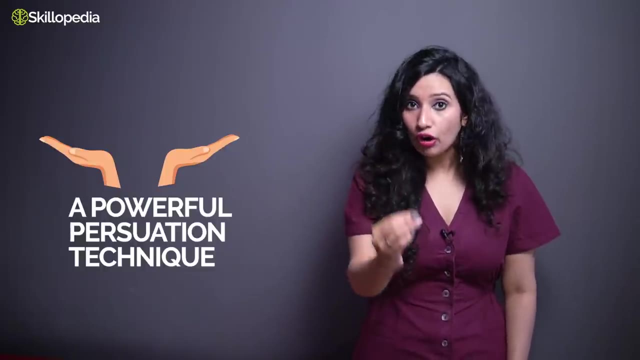 like listing. whenever you're contrasting different ideas, use your hands to show it. This is a powerful persuasion technique, which means it can persuade your audience to believe what you're saying is right, or to convince them of your opinion. So this can go well. 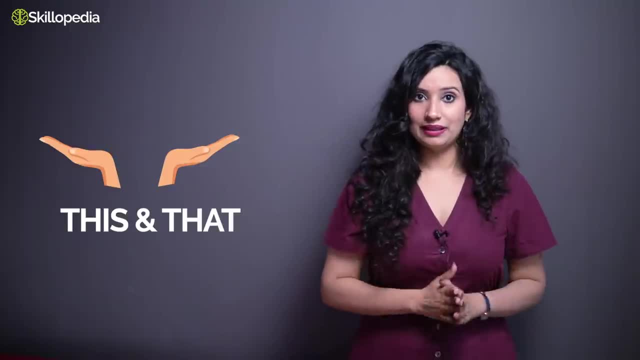 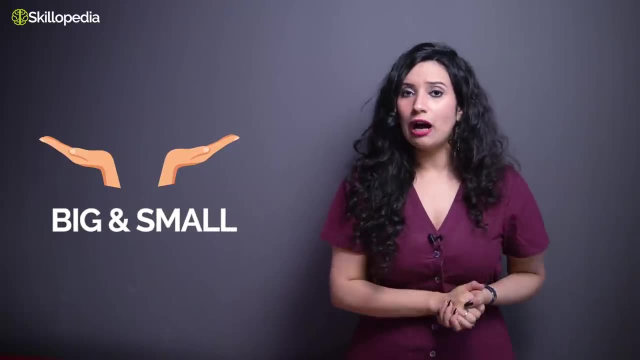 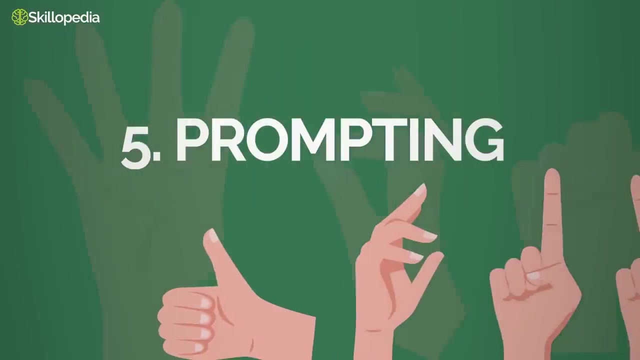 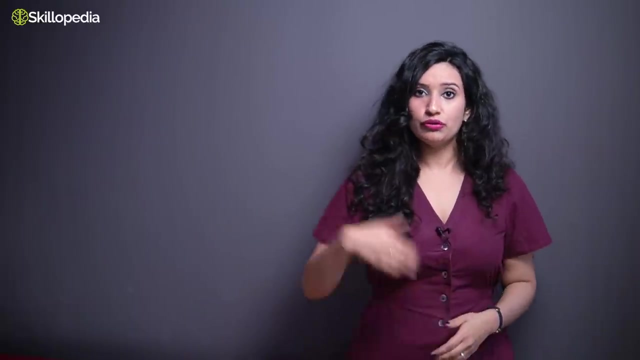 with this and that, or when you're talking about two different places. And there, what about the size, Big and small? I believe you've got the idea of how to use this hand gesture to separate two different things. Now to build on my previous point about engaging the audience. So you use your hands to engage. 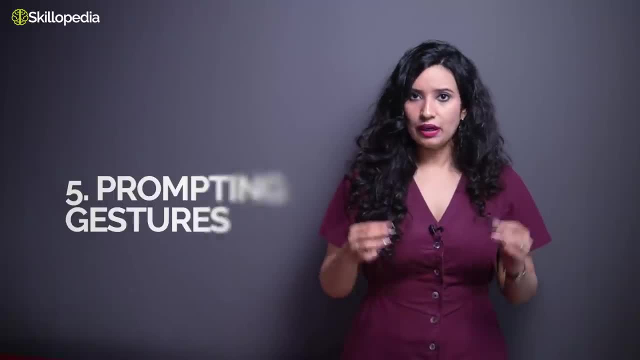 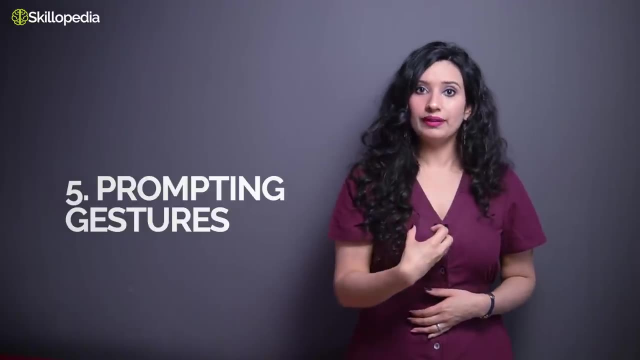 the audience. You can also use some prompting gestures. So you might wonder: what are prompting gestures? So these are those gestures that when you ask audience to do something, they do it along with them. So if you ask your listeners to raise their hand, you raise it. 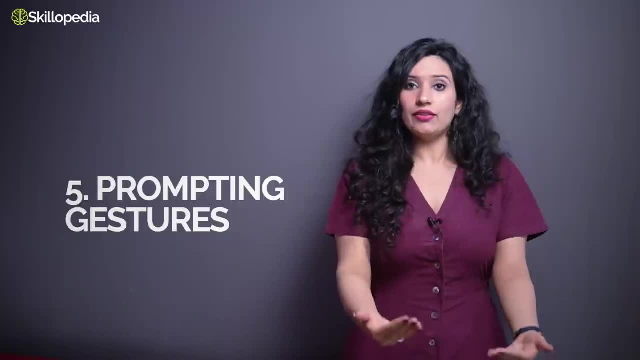 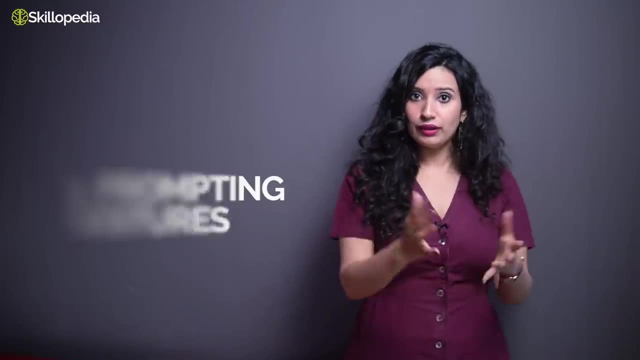 along with them. Or if you ask them to clap or perform any other action, you do it with them. So this is the reason. the reason you need to do this is to get them more engaged in your talk. For example, you might say: raise your hand if you want to earn million. 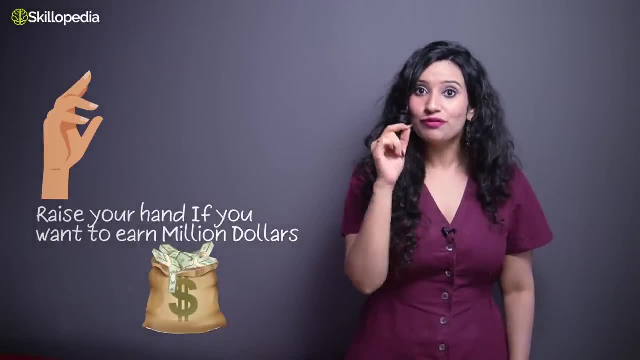 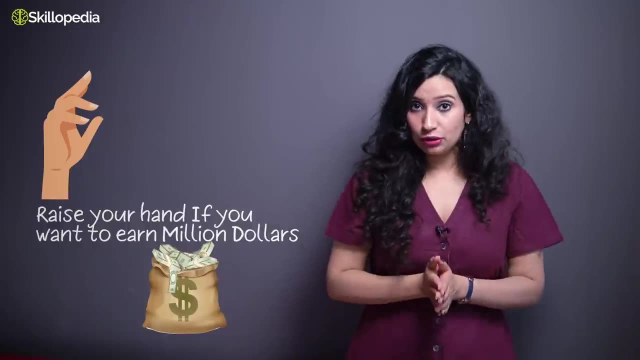 dollar this year. So when you say this, you should first raise your hand, because people and your audience will follow you right? This is because your audience is more likely to do it if they see you doing it, But if you don't do it, there's a high possibility.